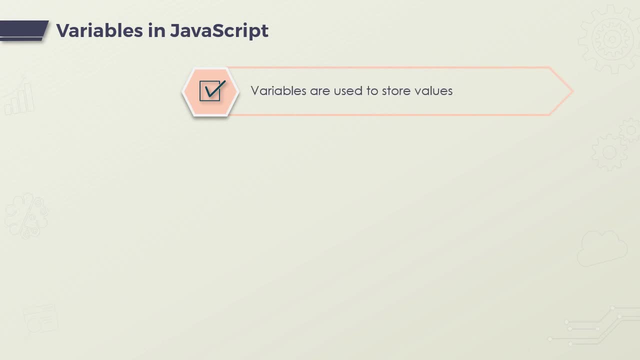 any other function in any other programming language. Variables are used to store values. That's it. Also, JavaScript natively supports three basic types. Now you may think that because it supports three basic types, it's not a full-fledged programming language, But there are. 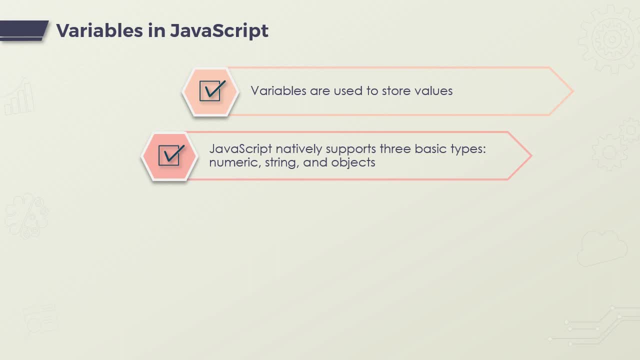 variations on these. So the basic ones are, of course, numeric string, where we use double quotation marks, and objects. Then we have constant variables. Now the constant variable type was not supported initially, But now recently with the last version of ECMAScript, so version 6,. 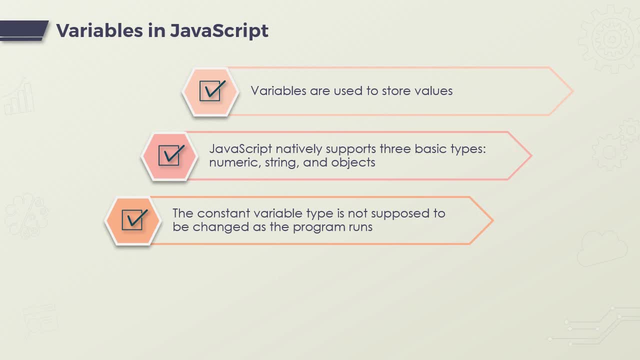 they did introduce the const variable type. So now we have a constant variable type that we can use, meaning that once we've declared a const, then the value that's inside of that variable cannot change during the running of the program. Literals work just like any other programming language. They are either numbers, strings, 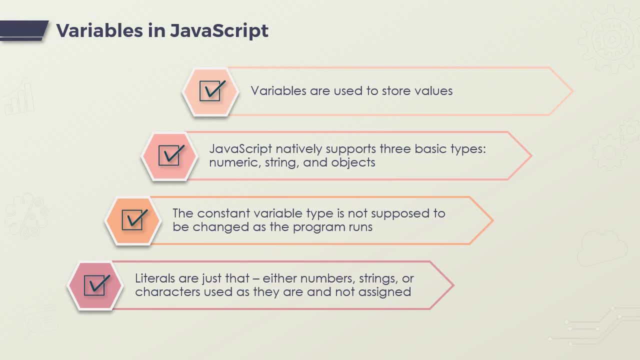 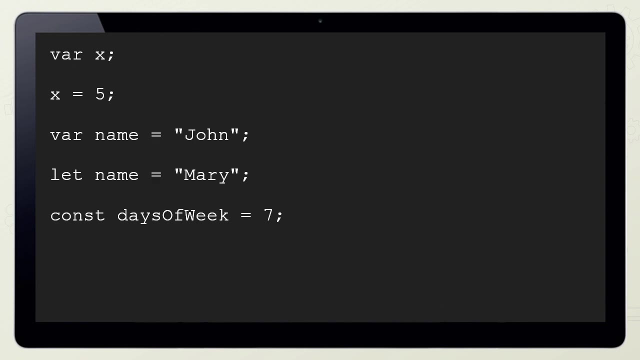 characters. Of course, strings are inside of double quotation marks And, just like any other programming language, literals are used, but they're not assigned to any variable as such. Let's take a look now at a short program in JavaScript And starting at line. 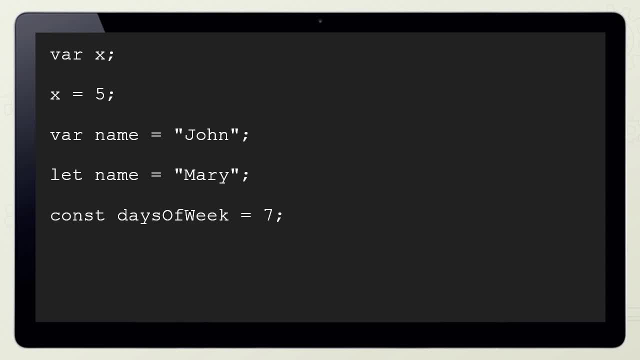 1, we see that we can declare a variable. All this means is that somewhere in memory, an address will be picked and that address will have a label of x in it. Later on, on line number 2, we can assign a value to that location. So in this case, on line 1,, we declare x. On line 2,. 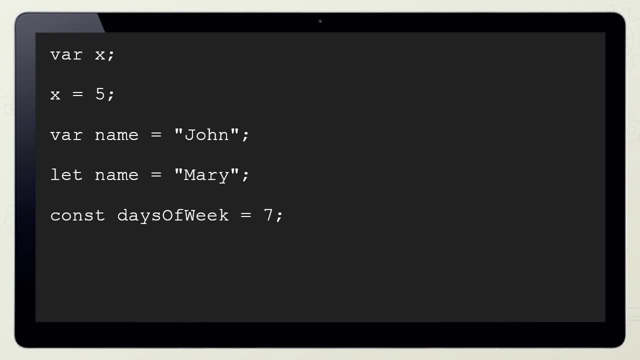 we initialize it with the value of 5.. On the third line, we've initialized, or we've declared and initialized a variable, a string variable, and then we've initialized it to the value of john. Then, further down, on line number 5, we've declared a value to the value of john And then we've initialized it to the value of john. 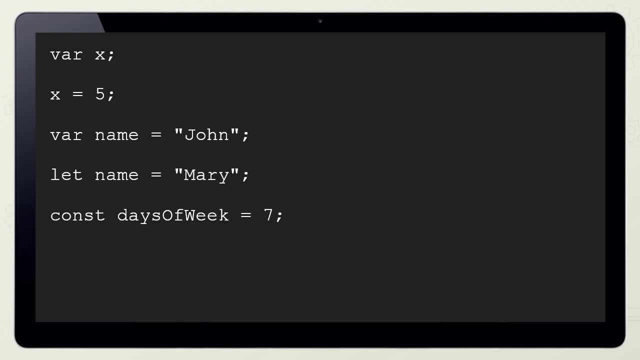 So on line 4, we've declared another variable and initialized it with a different word. Now you notice that there are two types of declarations here- var and let, And the difference has to do with scope. We will talk more about it when we get into the demos. So the vars are considered to be. 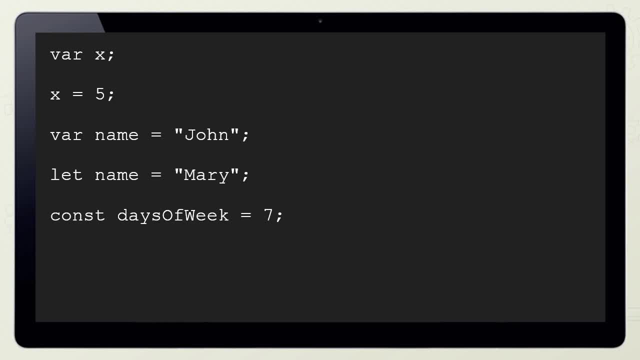 globally scoped, whereas the lets are considered to be scoped within the curly braces. And here, on line 5,, we see the cons that I previously mentioned. In this case, here, days of the week will be initialized with a value of john, And then we'll talk more about it when we get into the demos.